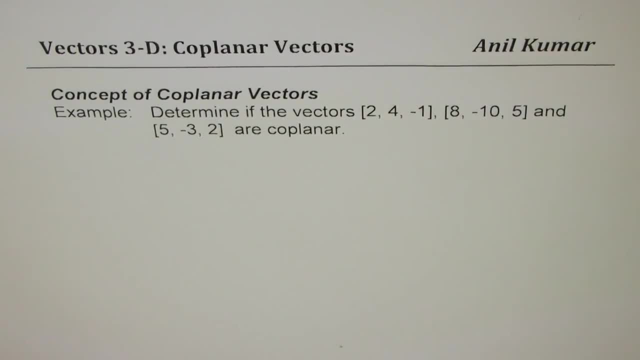 I'm Anil Kumar, sharing with you an excellent question from my subscriber, and I hope its solution will help many others Now. this question is on coplanar vectors. We'll first try to understand the concept of coplanar vectors and then take up this example which has been posted. 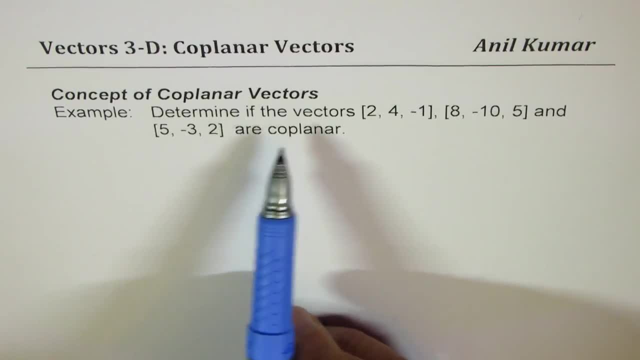 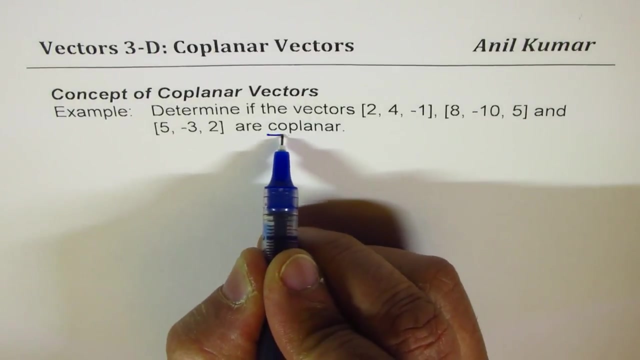 by our subscriber Determine if vectors 2, 4, minus 1,, 8, minus 10, 5 and 5, minus 3, 2 are coplanar. Now what do we understand by coplanar vectors? Let's understand the term coplanar first. 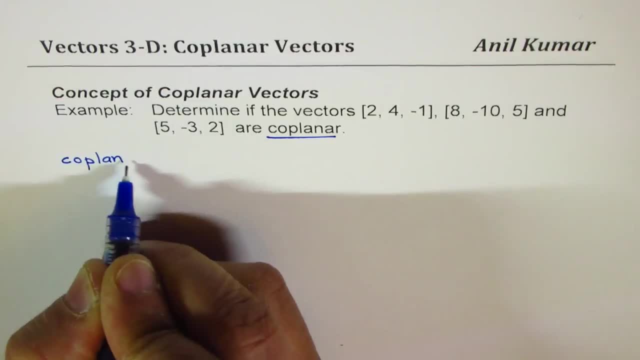 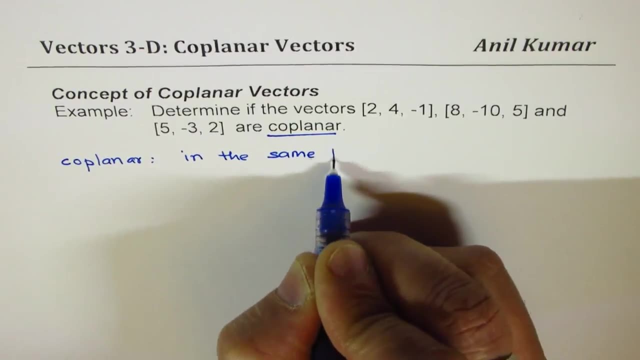 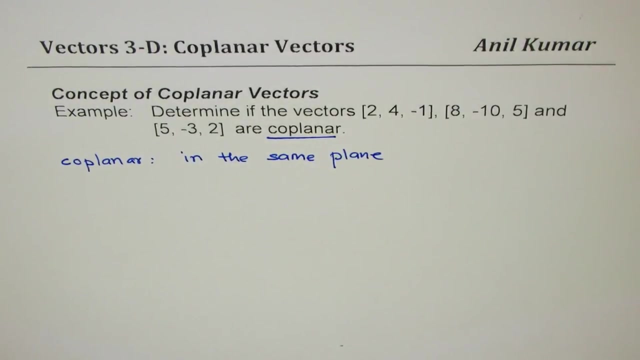 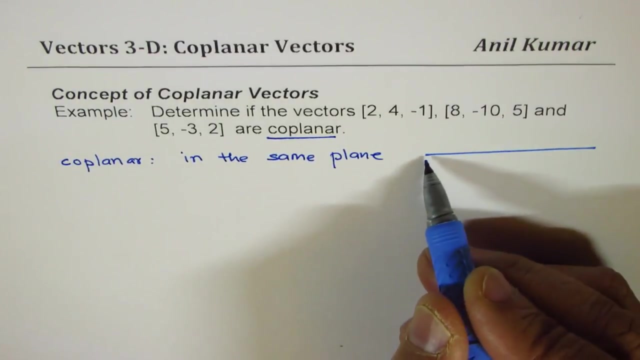 So coplanar means in the same plane, right? So coplanar means in the same plane. Now, let us say that these three vectors are coplanar. Let us say, let's assume, right, So? and then, if they are coplanar, let me say that they all, the three of them, could be represented. 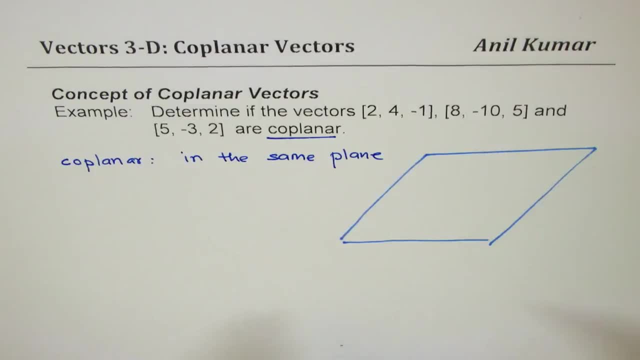 on this plane. That's the plane of this paper. okay, So we normally give the name of a plane by pi. That's the name which is very commonly used for naming planes. Now let me draw the three vectors here. Let's say, one vector is kind of like this, right The other. 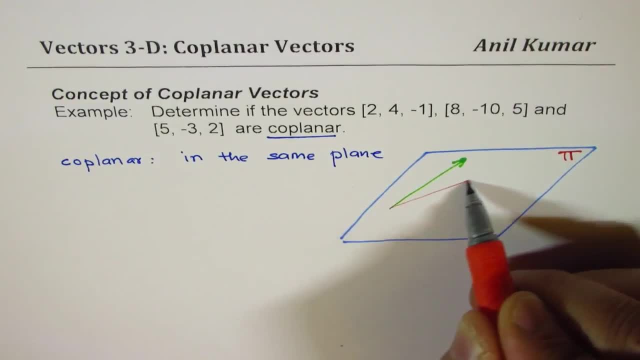 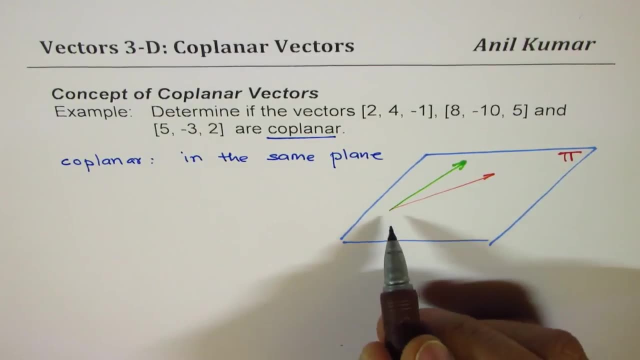 vector is kind of like this. And let me draw the third vector in a different ink. Let's say, the third vector is kind of like this: Well, I'm purposely drawing them with the tails at a common point. You can always, you know, place the vectors anyway, and that is all. You could always place them. 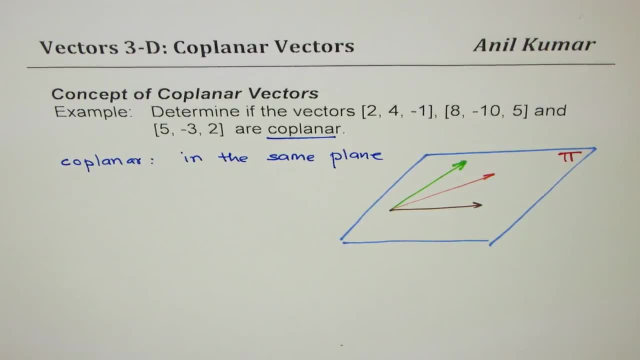 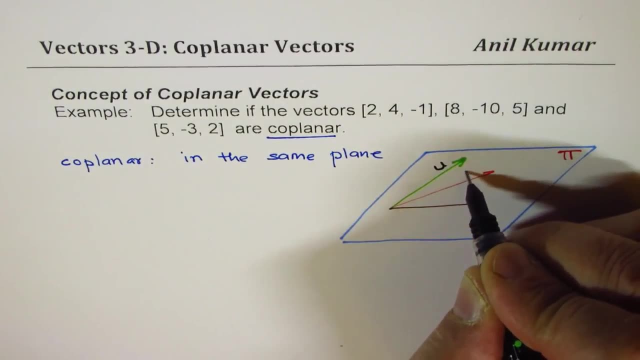 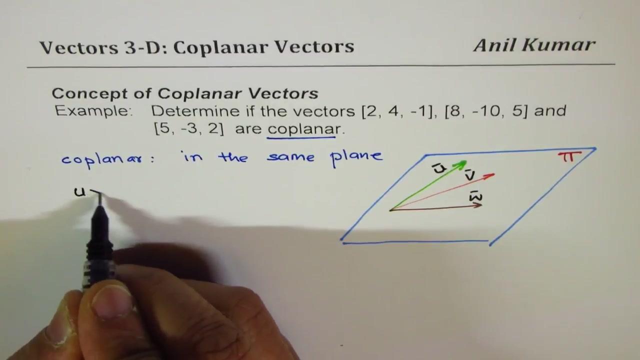 in the same plane right Now. see what happens when I do cross product of these vectors. Let's call them by the name: u, v and w. Let's say these are the three vectors. Now if I do u cross v. 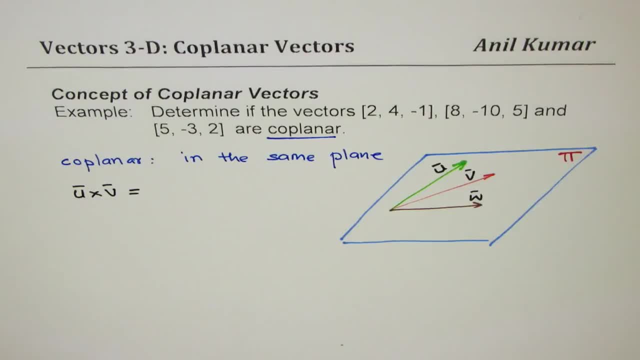 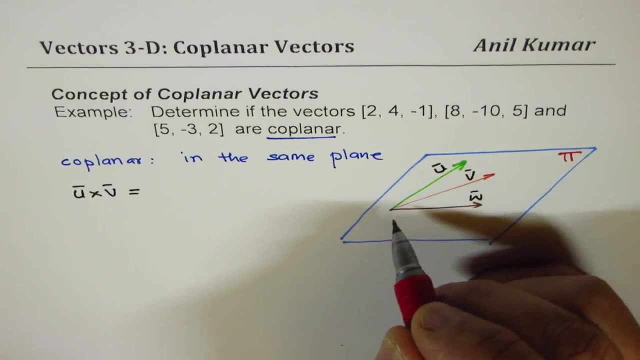 in that case, what will happen is that I will get a vector which is perpendicular to both of them, pointing outside or inside. So we'll assume that we are doing like this and like: screw over, So v cross u. I should have written, But anyway think as if it is going upwards, Is that okay? 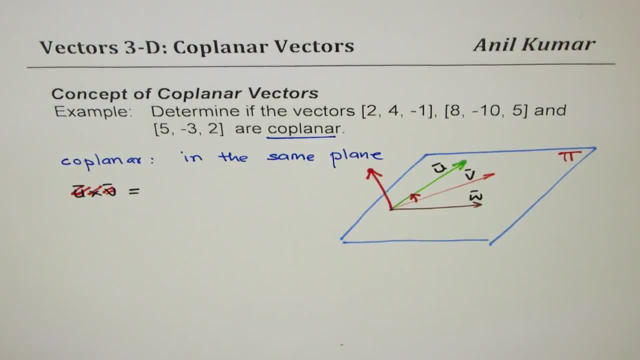 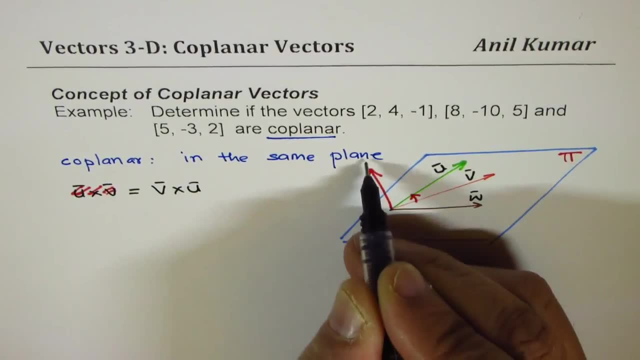 Right. So instead of let's be very specific. So if I, I will say I'll say v cross u, okay. So in that case the vector will be pointing outside and let's call this normal n, right So? 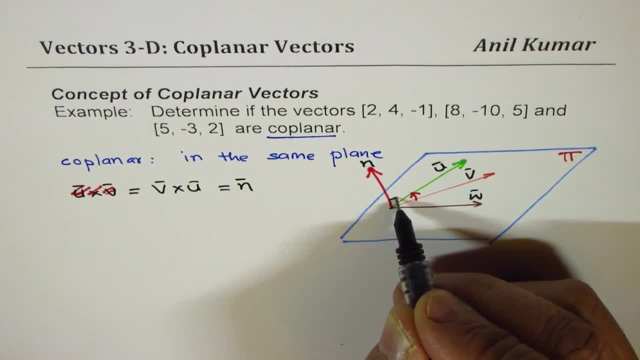 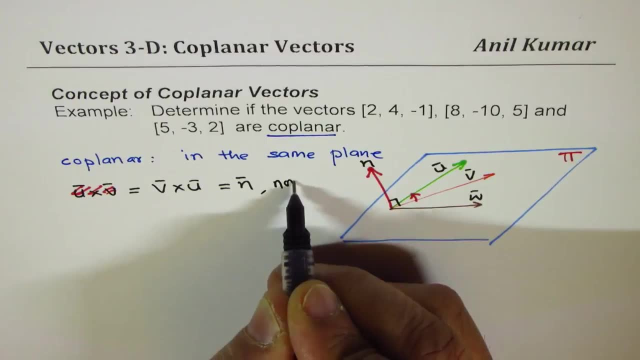 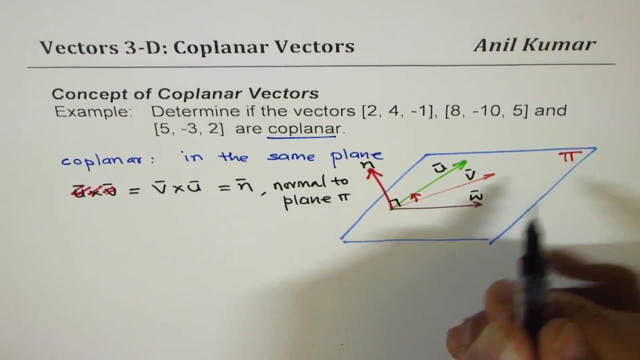 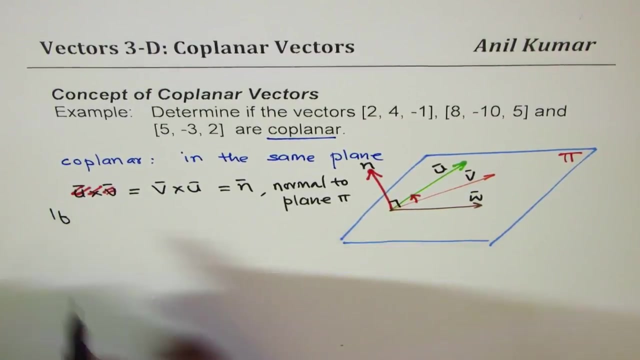 this is represented by vector n and this vector is going to be normal to both these vectors. It is normal to the plane pi, right, So n, which is normal to plane pi. So if it is normal to the plane pi, it is normal to each and every vector on this particular plane. Is that clear? Now we say: if this vector 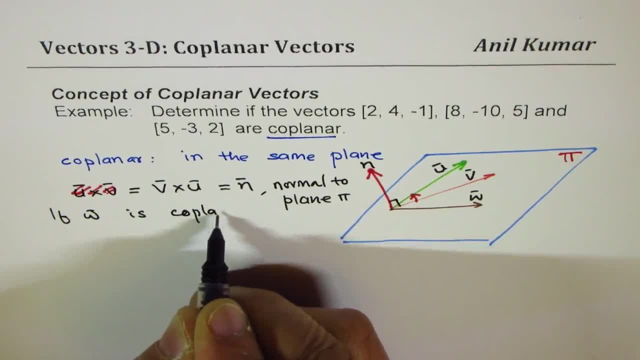 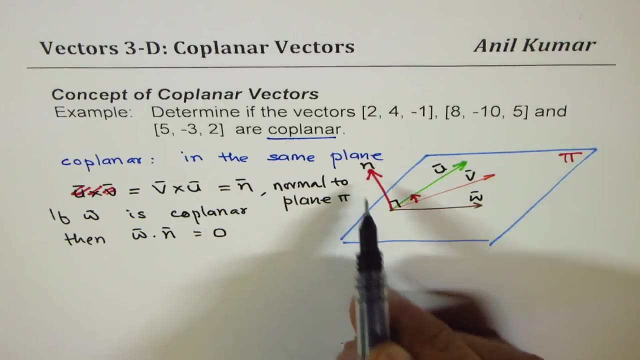 w is coplanar, then the dot product of W and n should be zero, right? Since normal vector is normal to the whole plane, it is normal to W also right? So we know cos 90 degrees is zero. So the dot product 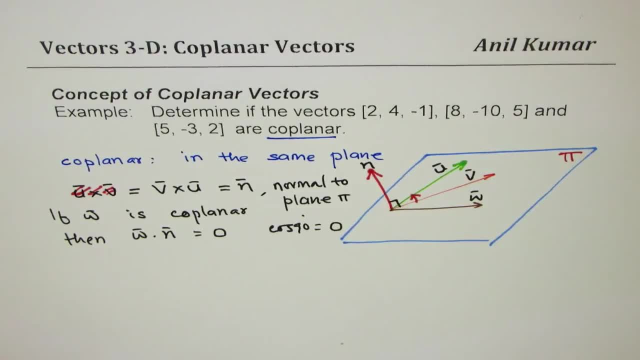 between W and n should be zero. Is that correct, Right? So what we did effectively is that we found scalar triple product, So we basically found the cross product of V and u and then dot product with the third vector. Is that okay? And if that is equal to zero, 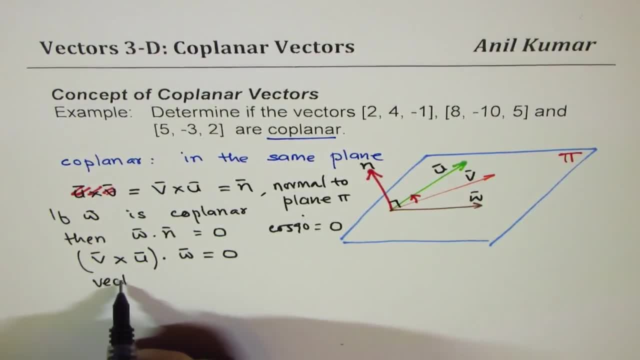 then we say that the vectors are coplanar, correct. So that becomes a condition for any three vectors to be Coplanar. Is that clear, Perfect? So I will call this as one way of doing it. So let 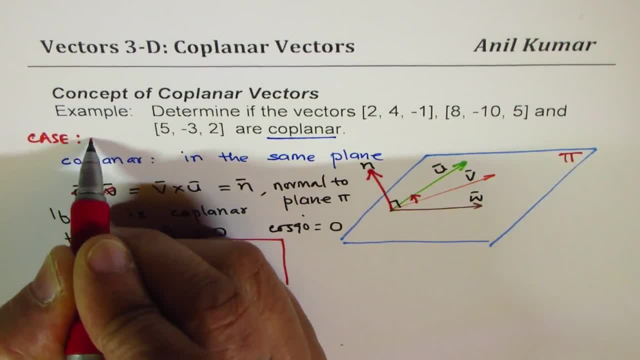 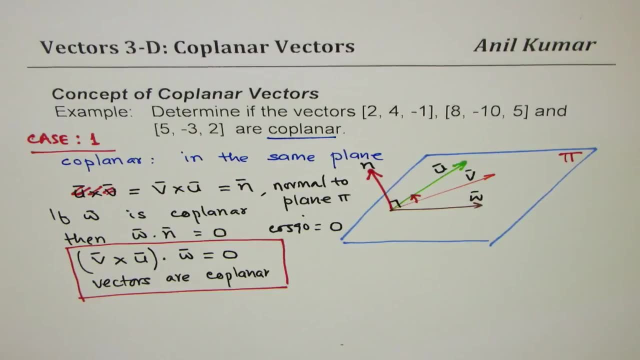 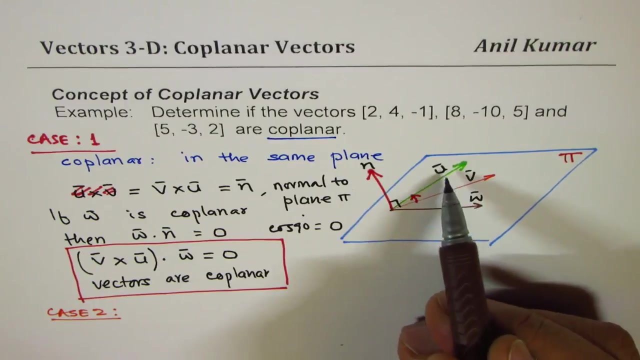 me say: this is case one, Okay, This is case one for us. Case two, which I will also discuss in this particular video, is that let me write down case two: Okay. Case two is that, in case they all are coplanar, then I could write one vector as: 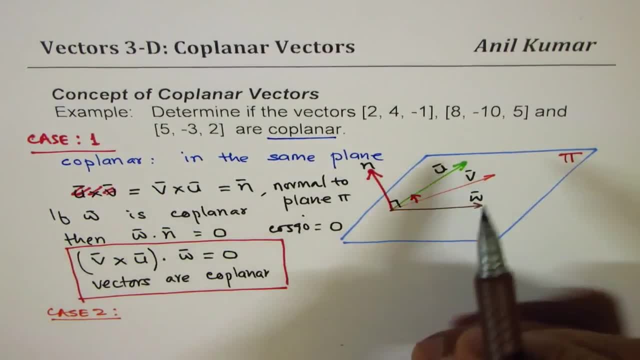 a combination of other two right? So, for example, I could represent vector V as combination of these two. correct Making a parallelogram. So if I choose to represent V as a combination of these two, one way could be like this. Let me show you here. So if I draw a vector parallel to 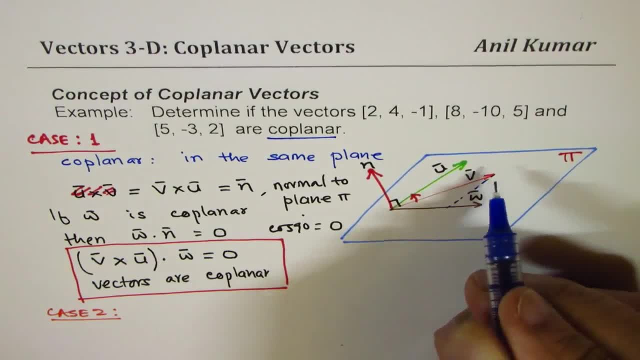 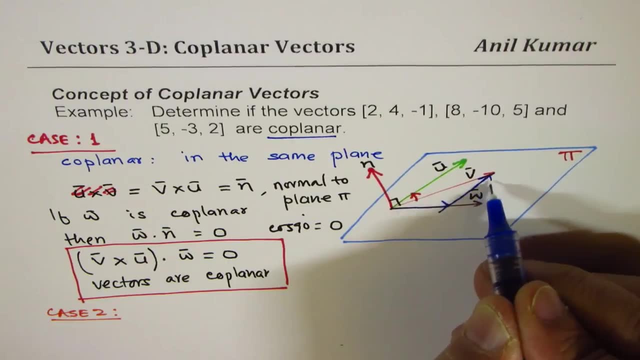 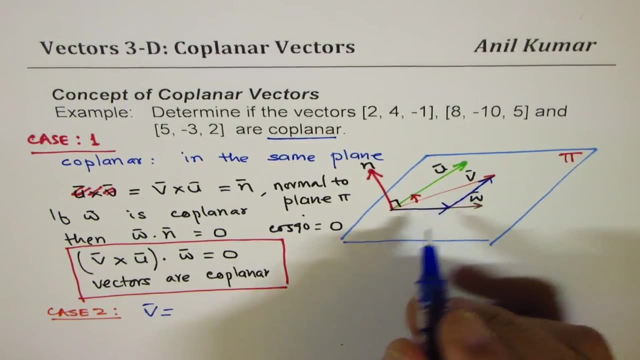 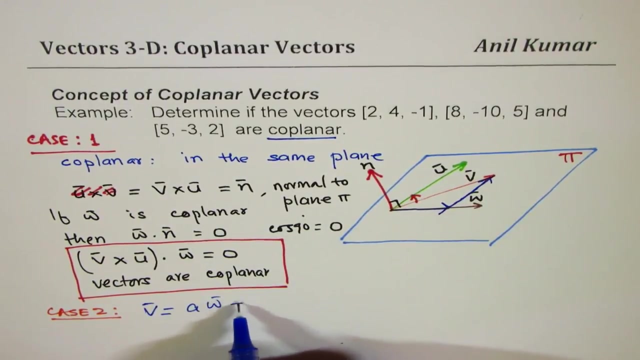 this kind of like this, is it okay? In that case, scalar multiple of w and scalar multiple of u could be equal to v, right? So I could represent vector v as combination of these two. That is to say, a times this becomes scalar multiple of w, plus b times scalar multiple of u, You get an. 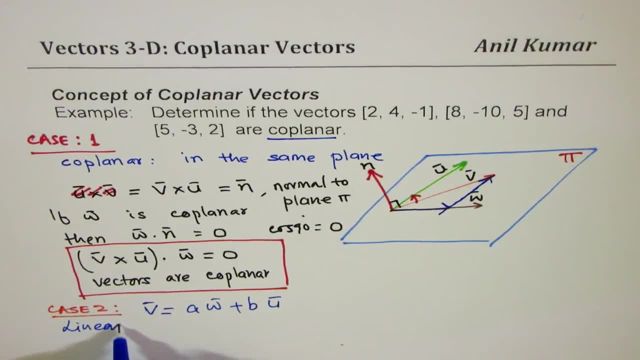 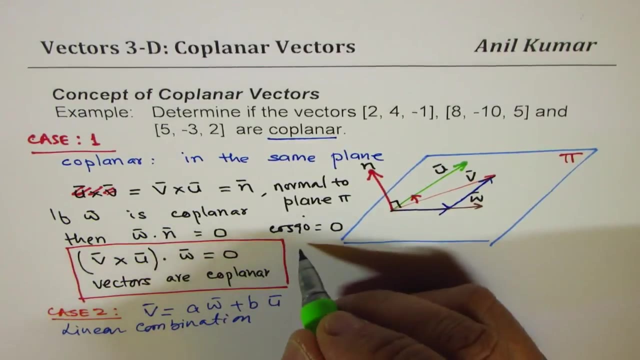 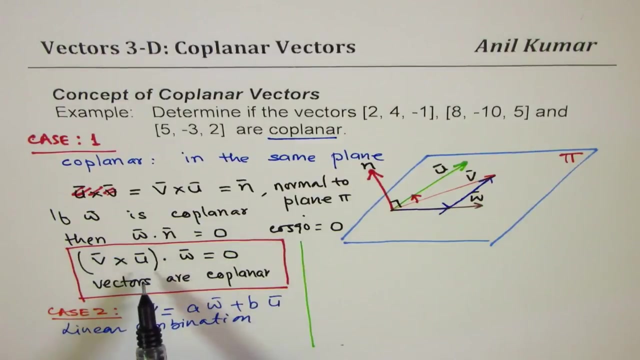 idea right. So that is a linear combination. So this is another way of showing that the three vectors are coplanar. Perfect, So that is how you could actually explain about the coplanar vector, Correct? Now in this space, I will do the first part, which is we'll find the scalar triple. 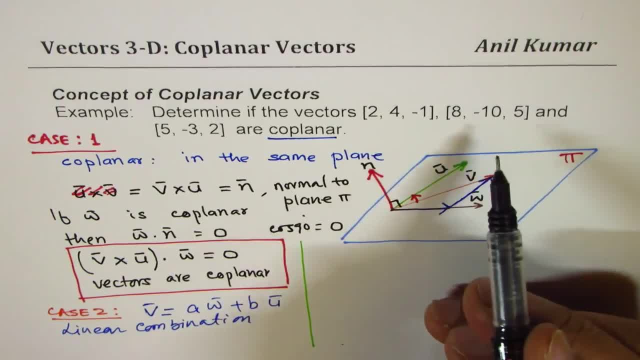 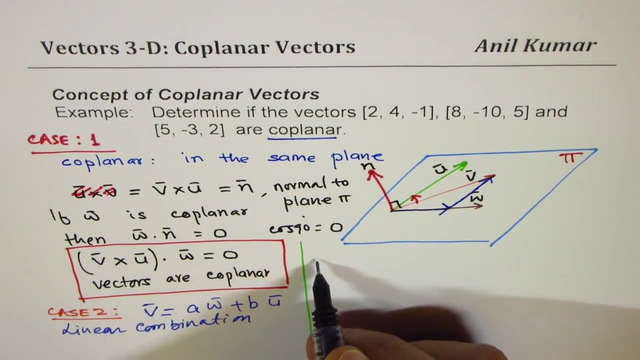 product of these vectors. And then in the next page, in the same video of course, I will show you how we can write one vector as a combination of other two. Correct, So let's do the triple product, So we can do all of these three things together. So we write this as 2,, 4,. 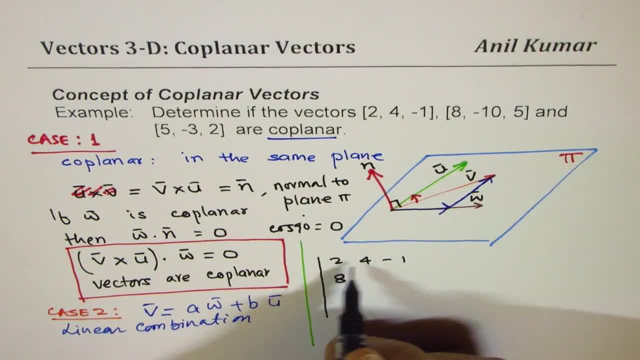 minus 1, times. so we'll do dot product with this of cross product, with 8 minus 10, 5, and 5 minus 3, 2.. Correct, So I'll use this space to calculate. So it is 2 times minus 10 times 2,, which is minus. 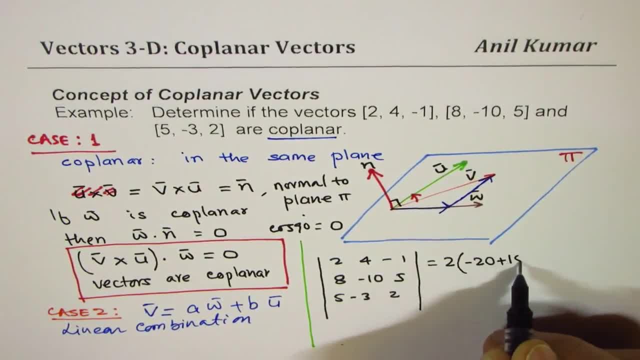 20. Minus this, that is plus 15.. Minus 4 times 8 times 2 is 16.. 5 times 5 is 25, minus 25.. And then we have a minus. let me write minus one time: 8 times 3 is: 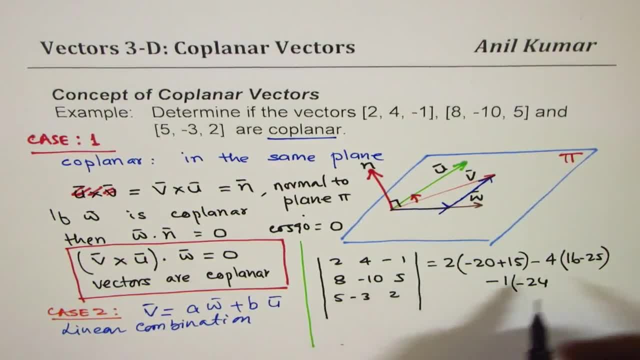 24, which is a negative sign here, And minus of this gives me positive 50. Correct, Okay. So if you calculate, you get 2 times minus 5.. And here you get minus 4 times 9, right, negative 9.. Okay. 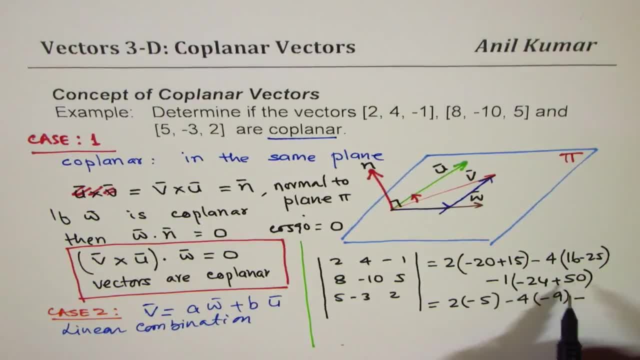 And this is a minus 20,, this is minus 26.. Correct, And that gives you minus 10.. And that is minus, minus is plus 36.. And this is minus 26.. And that is indeed 0. Since scalar triple product is 0, correct? We? 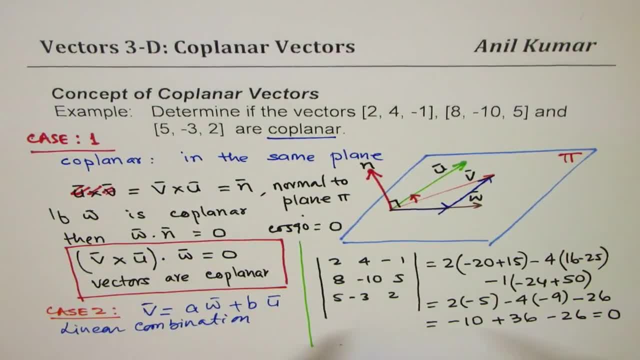 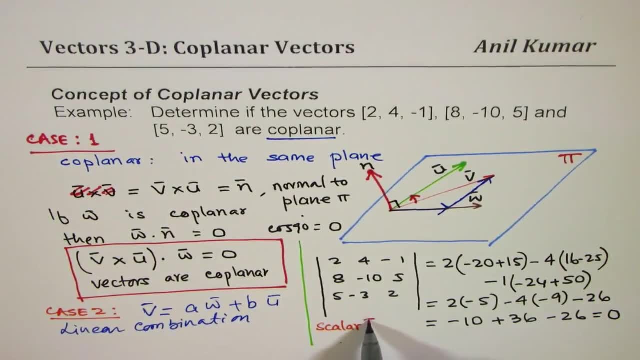 can write that these vectors are coplanar, right? So that means, since we got that scalar triple is 0,, right, And that means they are coplanar. Is that okay? So that is very important. Now. 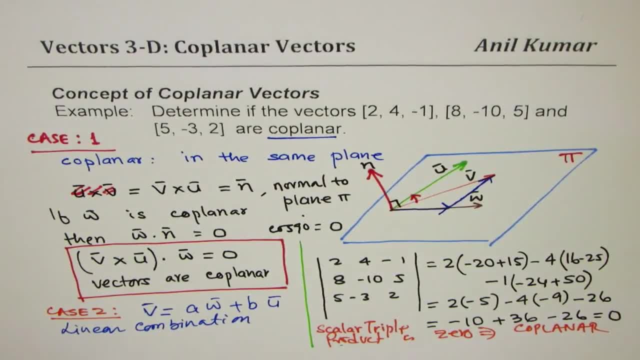 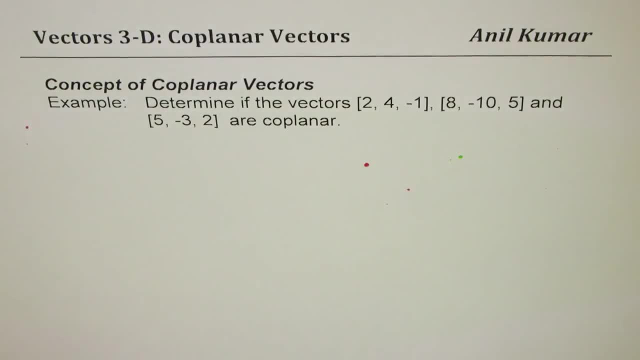 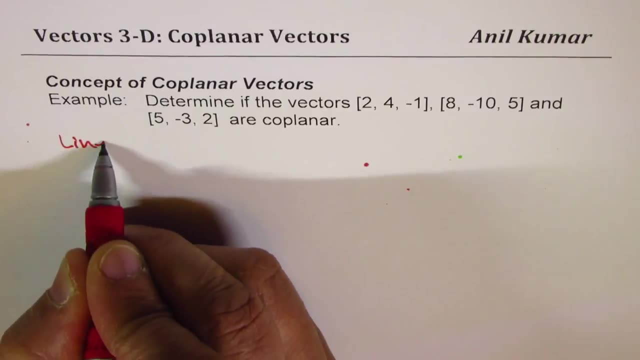 we know they are coplanar, But now it's a good idea to write one vector in the as a sum of other, two rather linear combination, right? So let's look into that part now. So in this case, again I've copied the same question. I will write one as a linear combination. 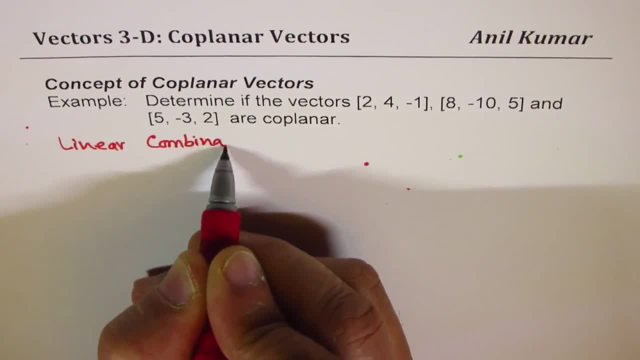 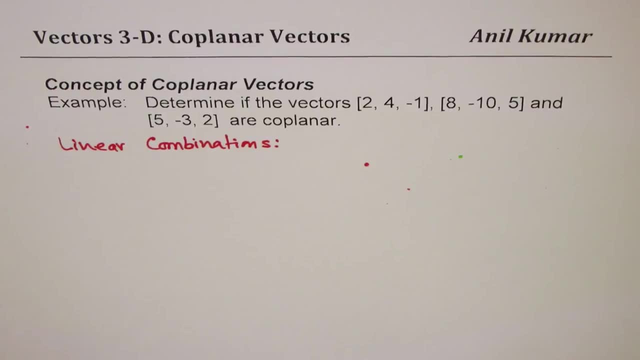 of others. Okay, So you could use any one of these methods. You don't have to do both, But I'm not sure which one has been taught to you. right, So do the one which is better for you. Correct, So a linear combination really means that we have to write one vector as a combination of: 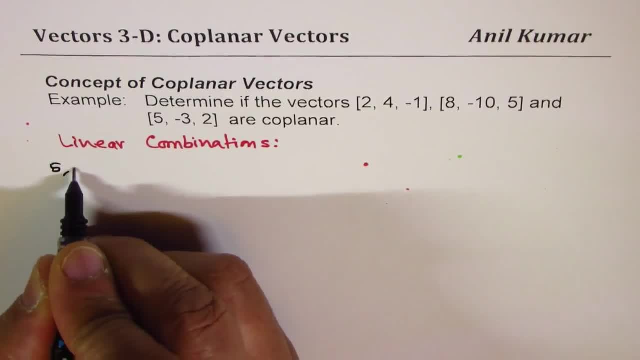 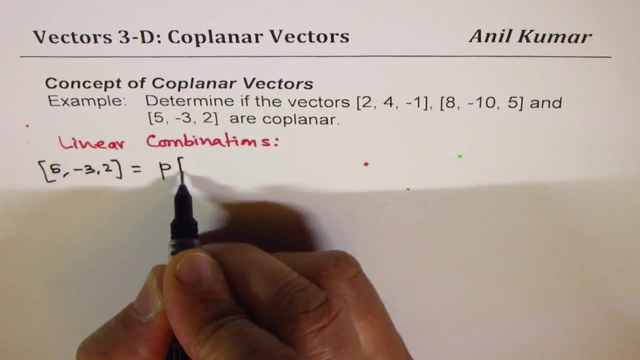 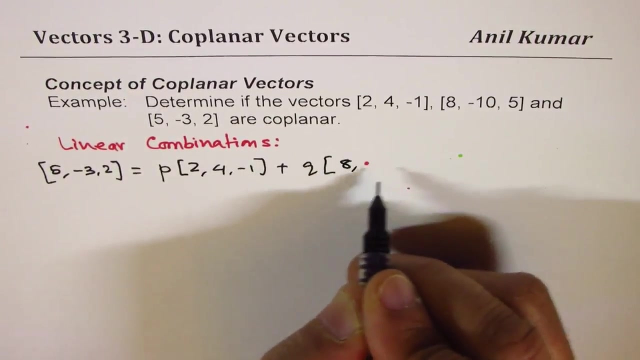 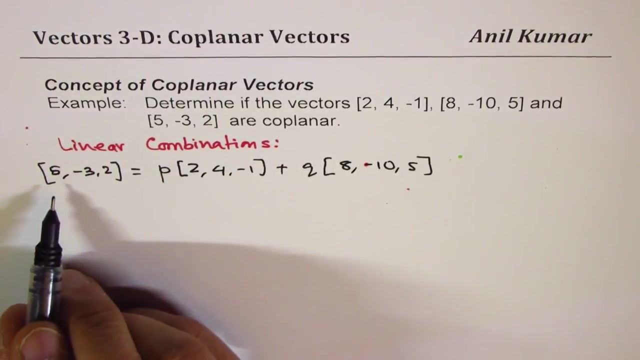 rather two. So we let's write 5 minus 3, 2 as a combination of these two vectors, Let's say p times 2, 4 minus 1 plus q times. let's say 8 minus 10, 5. Correct, So if you expand you could. 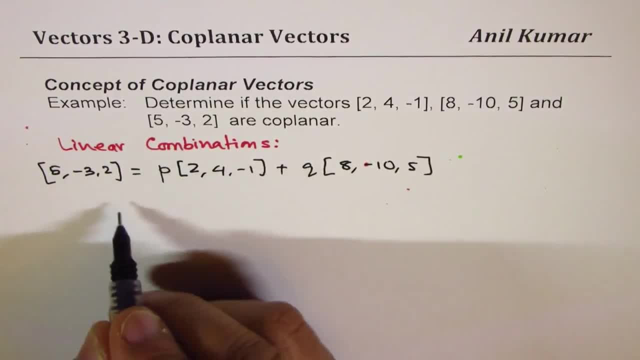 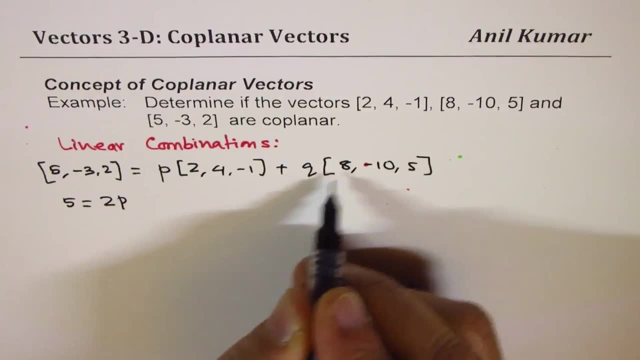 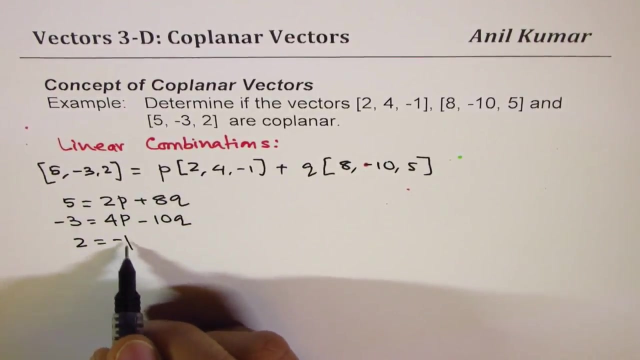 get direction numbers a, b and c for each right So we could write: we get three equations from here. One is: 5 equals to 2p plus 8q minus 3 equals to 4p minus 10q And 2 equals to minus p. 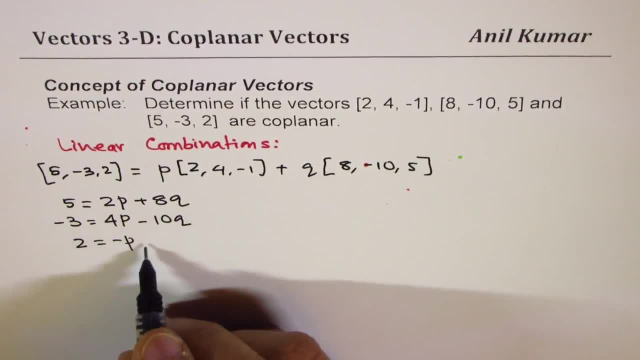 And here we get 5q. Perfect. Okay Now from the last equation, I could write p as equal to. I could write p as equal to. if I bring p this time, it is 5p minus 2. Perfect. So I have related one in terms of the other. 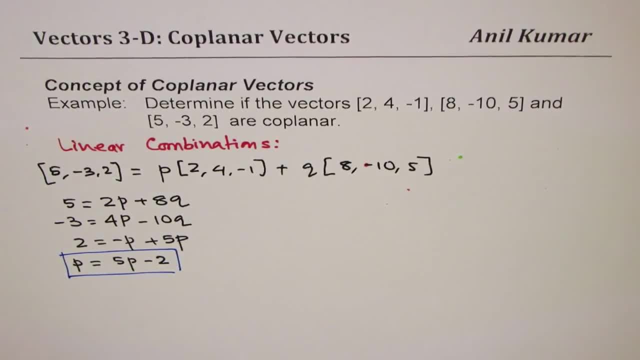 p as equals to 5p minus 2.. So I could substitute in one of our equations- Let me call these equations as equation 1,, 2, and 3.. Okay, And this is my equation 4.. So I'm substituting p equals to 5,. I mean 5q, I mean, what did I do? 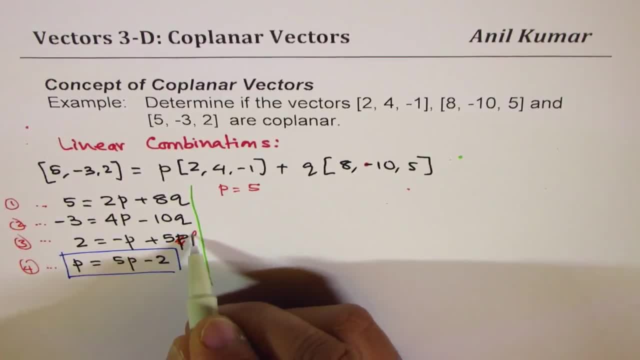 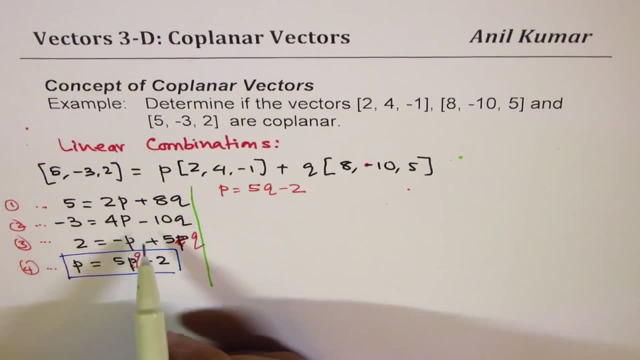 Okay, So it is q, not p, right 5q. Okay, So I'm substituting p equals to 5q minus 2 in one of our equations. Let me do it in 2, in 1.. Okay, So 4 in 1.. 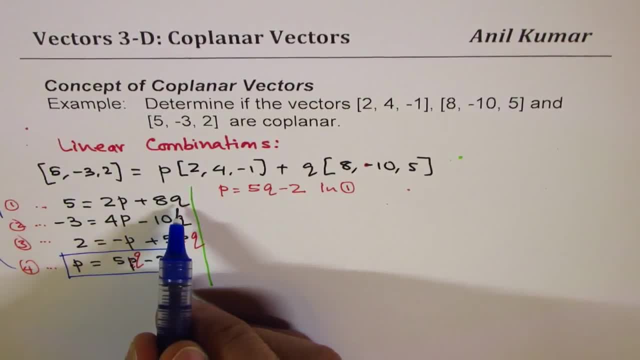 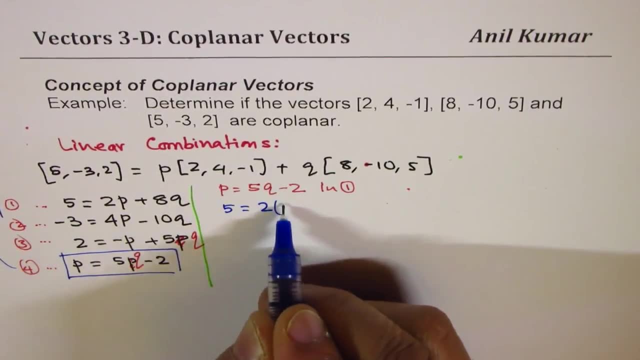 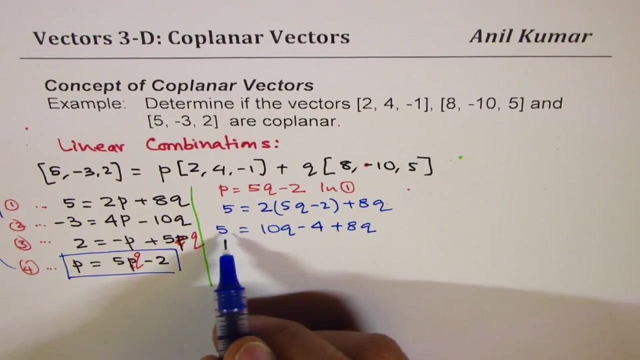 So this value here and then we'll find what what Q is. so we have this equation as 5 equals to 2 times P. so instead of P I'm writing 5 Q minus 2 plus 8 Q. so that gives me 5 equals to 10 Q minus 4 plus 8 Q. or bringing this 4 to this side, we get 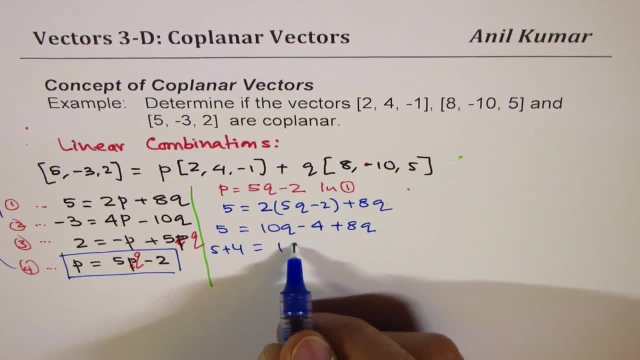 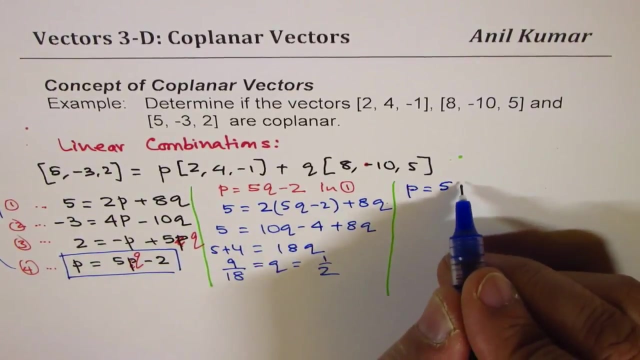 5 plus 4 equals to 10 plus 8, which is 18 Q, or 9 divided by 18 is Q, so we get Q value is half, okay. so if Q is half, what is P equals to? let's calculate so: P is equals to 5 times 5 times Q, which is half minus 2, and that gives you.